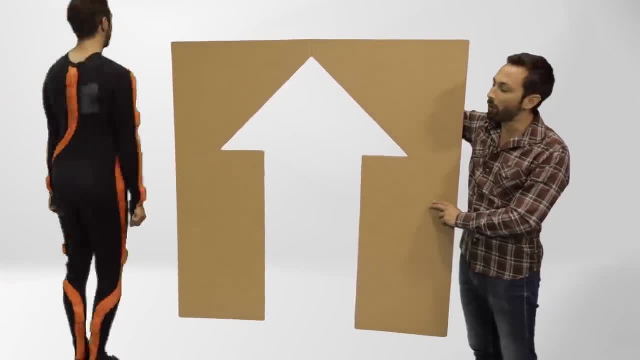 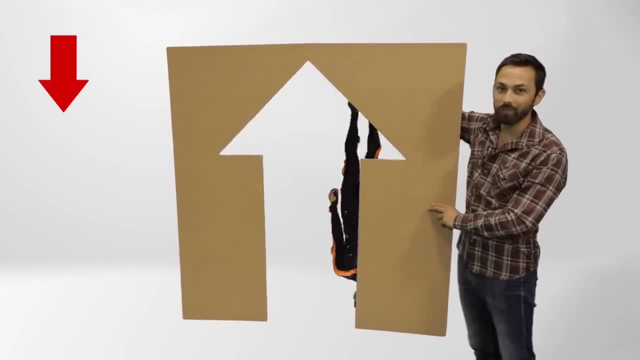 And this measurement can have only one of two outcomes: Either the particle's spin is aligned with the direction of measurement, which we'll call spin up, or it is opposite, the measurement which we'll call spin down. Now, what happens if the particle's spin is vertical but we measure its spin horizontally? 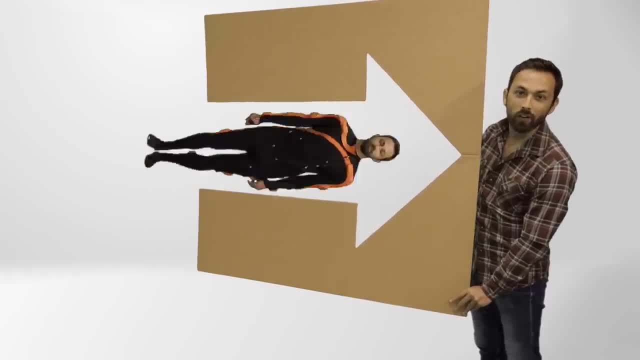 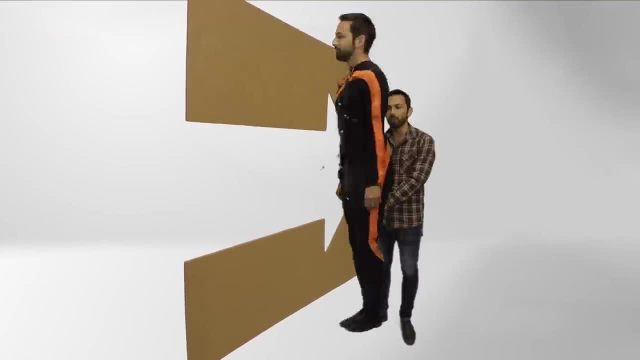 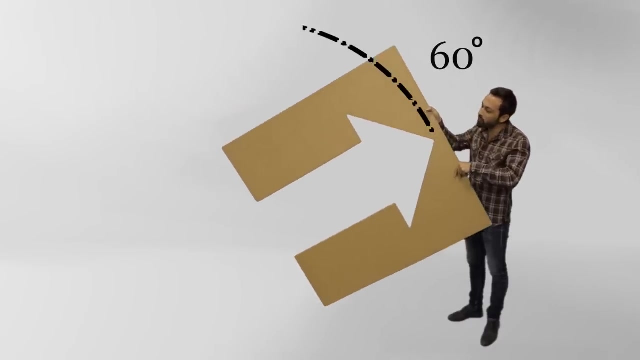 Well then, it has a 50% chance of being spin up and a 50% chance of being spin down, And after the measurement the particle maintains this spin. So measuring its spin actually changes the spin of the particle. What if we measure spin at an angle 60 degrees from the vertical? 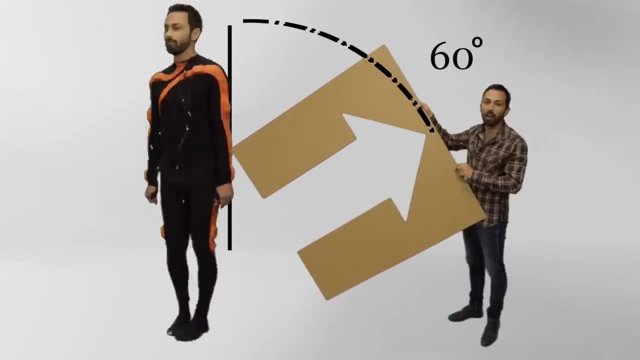 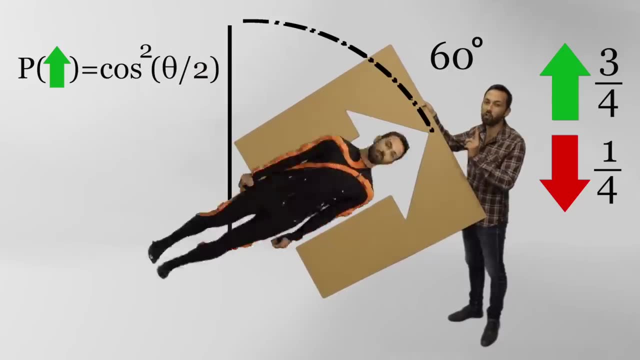 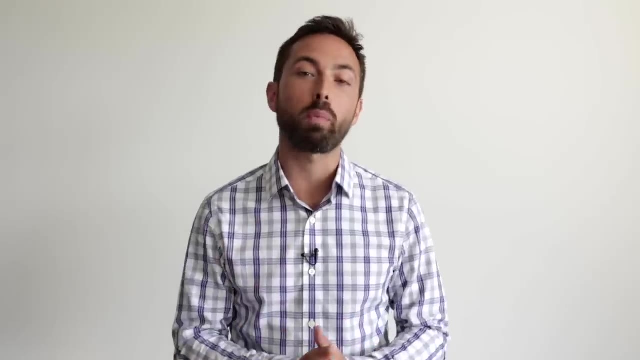 Well now, since the spin of the particle is more aligned to this measurement, it will be spin up three quarters of the time and spin down one quarter of the time. The probability depends on the square of the cosine of half the angle. Now, an experiment like the one Einstein proposed can be performed using two of these particles. 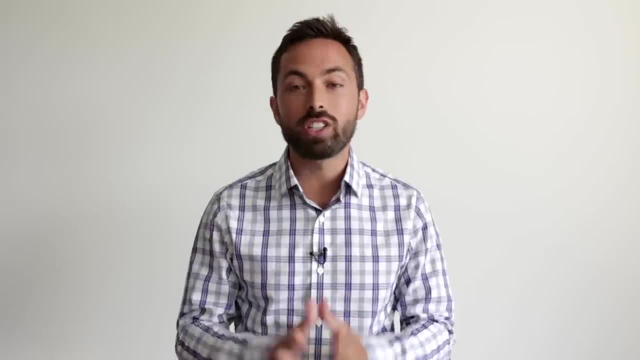 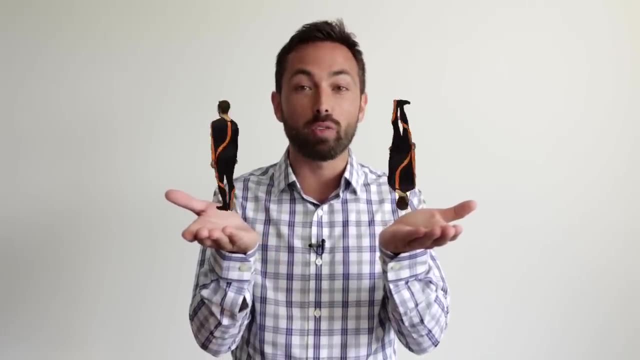 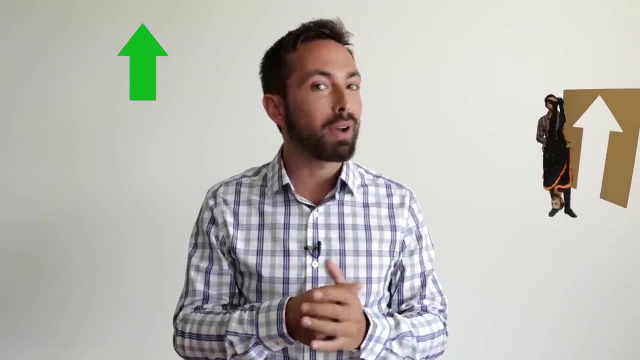 but they must be prepared in a particular way, For example, formed spontaneously out of energy. Now, since the total angular momentum of the universe must stay constant, you know that if one particle is measured to have spin up, the other measured in the same direction must have spin down. 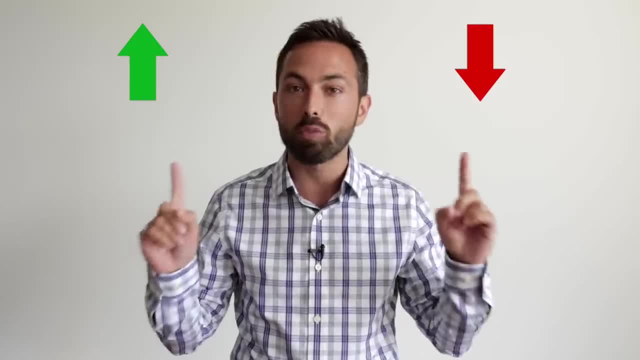 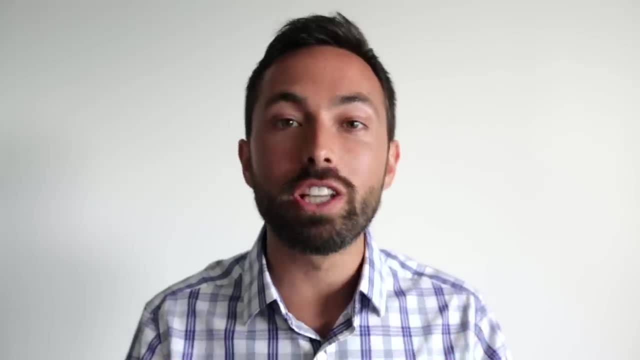 I should point out, it's only if the two particles are measured in the same direction that their spins must be opposite. Now here's where things start to get a little weird. You might imagine that each particle is created with a definite, well-defined spin. 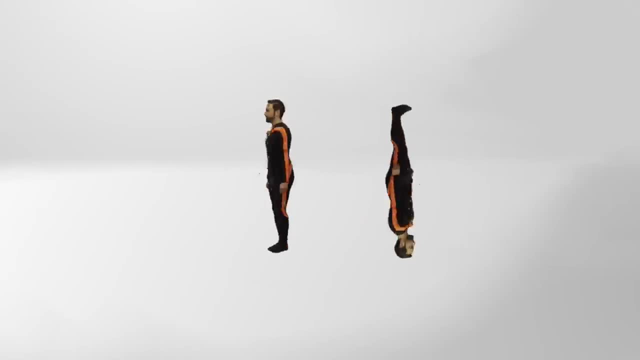 But that won't work, and here's why. Imagine their spins were vertical and opposite. Now, if they're both measured in the horizontal direction, each one has a 50-50 chance of being spin up. So there's actually a 50% chance that both measurements will yield the same spin outcome. 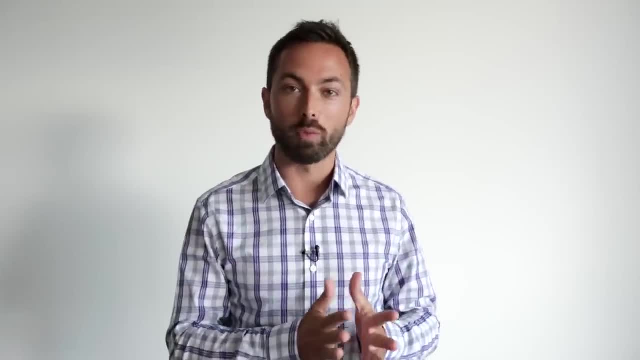 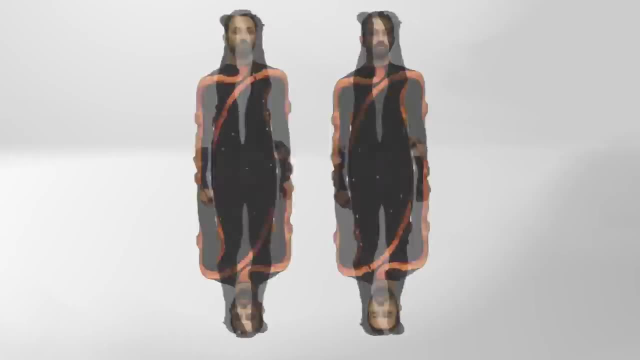 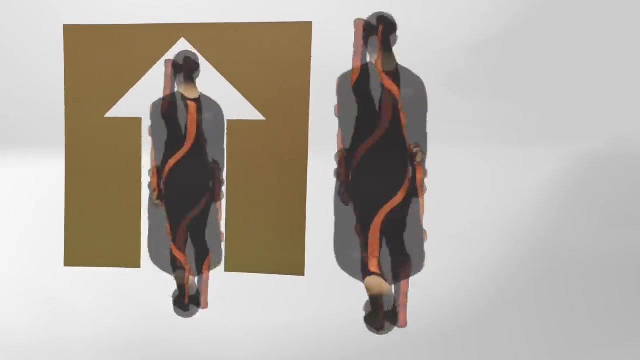 And this would violate the law of conservation of angular momentum. According to quantum mechanics, these particles don't have a well-defined spin at all. They are entangled, which means their spin is simply opposite that of the other particle. So when one particle is measured and its spin determined, you immediately know what the same measurement of the other particle will be. This has been rigorously and repeatedly tested experimentally. It doesn't matter at which angle the detectors are set or how far apart they are. they always measure opposite spins. Now just stop for a minute and think about how crazy this is. 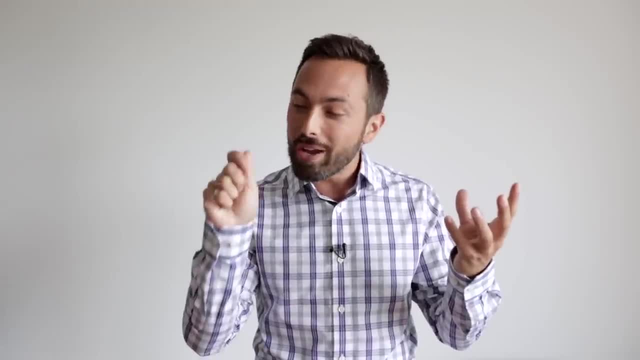 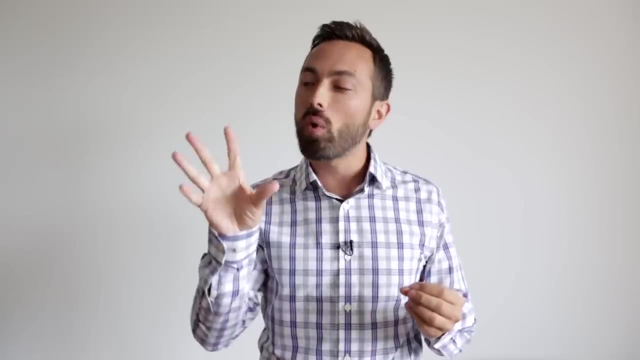 Both particles have undefined spins, and then you measure one and immediately you know the spin of the other particle, which could be light-years away. It's as though the choice of the other particle over the first measurement has influenced the result of the second. 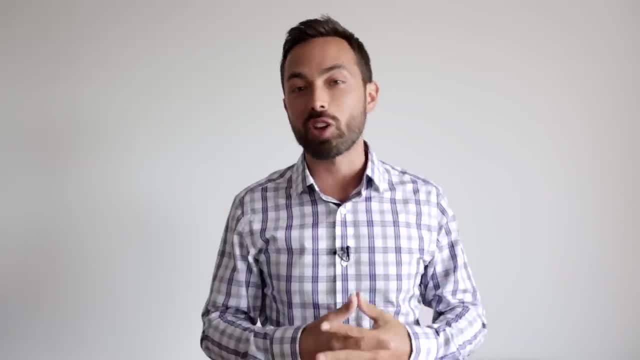 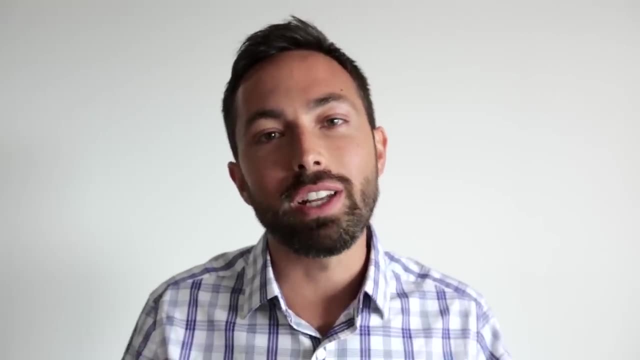 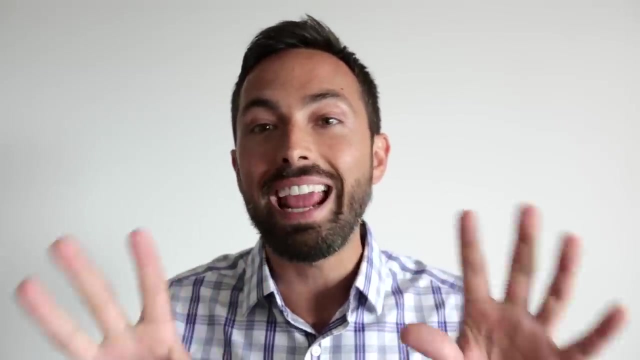 faster than the speed of light, which is indeed how some theorists interpret the result, But not Einstein. Einstein was really bothered by this. He preferred an alternate explanation: that all along, the particles contained hidden information about which spin they would have if measured in any direction. 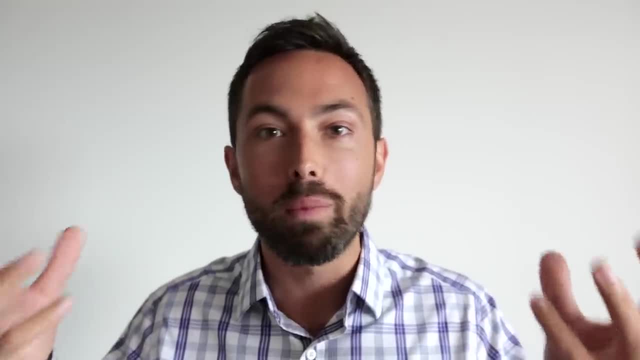 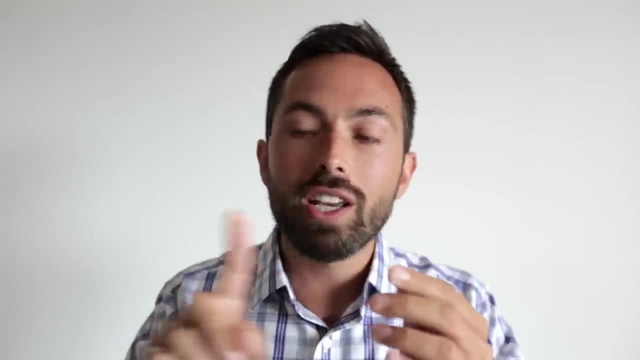 It's just that we didn't know this information until we measured them. Now, since that information was within the particles from the moment they formed, at the same point in space, no signal would ever have to travel between the two particles faster than light. Now, for a time, scientists accepted this view. 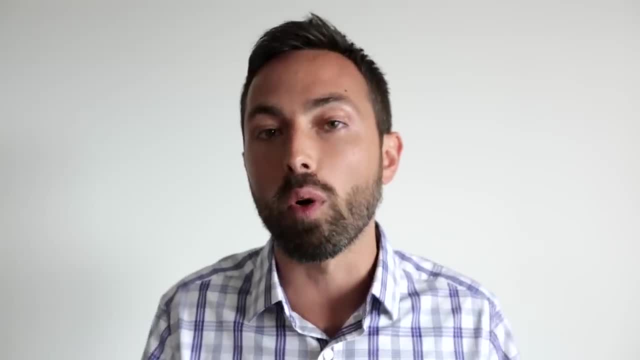 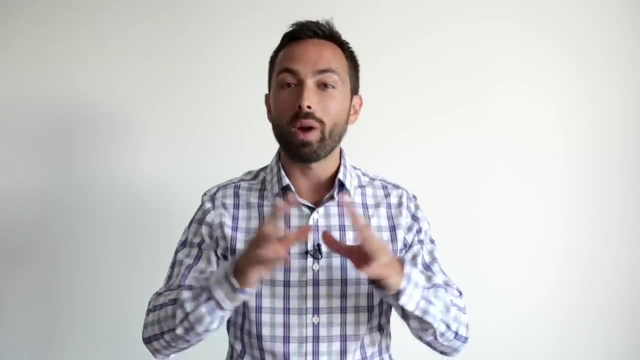 that there were just some things about the particles we couldn't know before we measured them. But then along came John Bell with a way to test this idea. This experiment can determine whether the particles contain hidden information all along or not, And this is how it works. 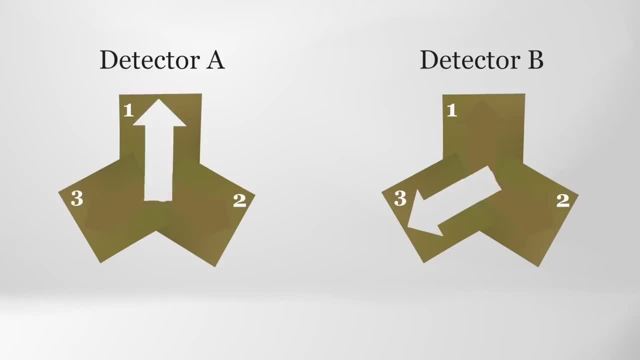 There are two spin detectors, each capable of measuring spin in one of three directions. These measurement directions will be selected randomly and independent of each other. Now pairs of entangled particles will be sent to the two detectors and we record whether the measured spins are the same. 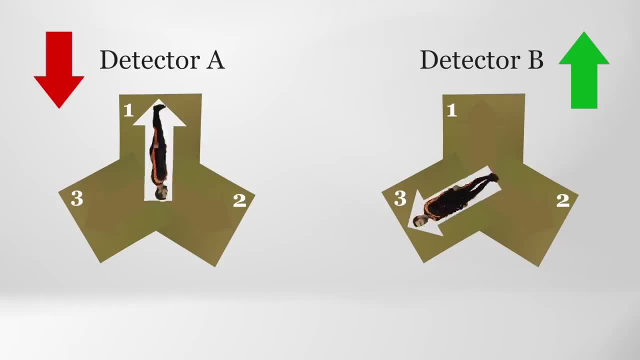 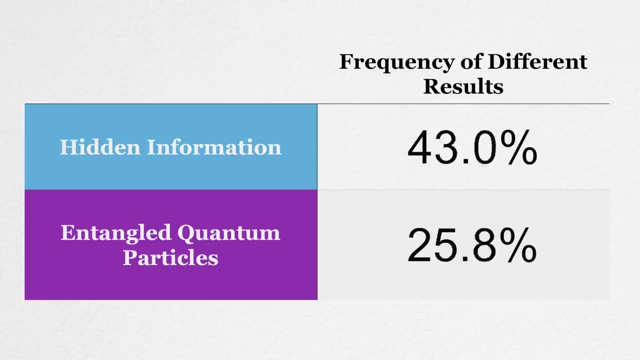 both up or both down, or different. We'll repeat this procedure over and over, randomly varying those measurement directions to find the percentage of the time the two detectors give different results. And this is the key, because that percentage depends on whether the particles contain hidden information all along. 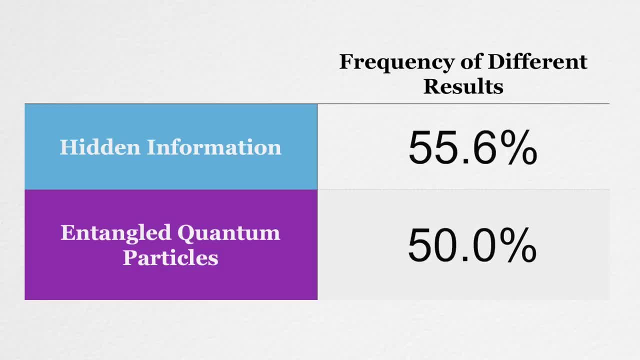 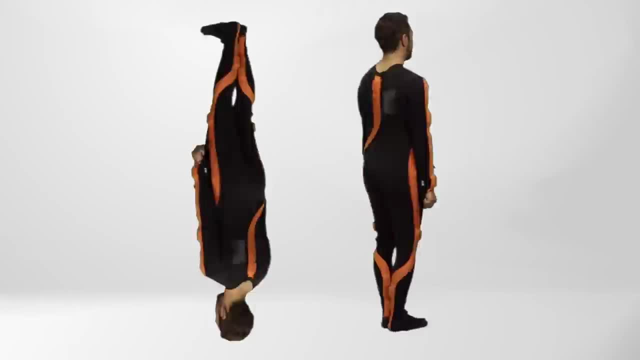 or not, Or if they don't. Now to see why this is the case, let's calculate the expected frequency of different readings, if the particles do contain hidden information. Now you can think of this hidden information like a secret plan the particles agree to. 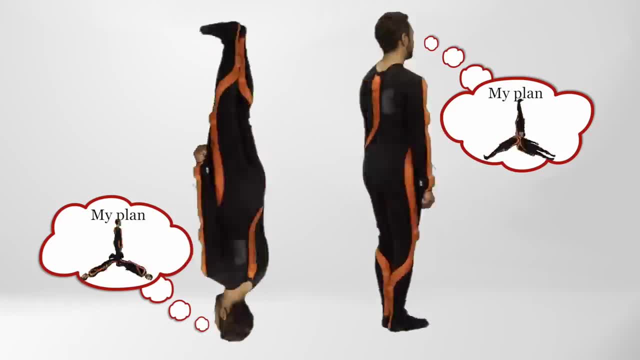 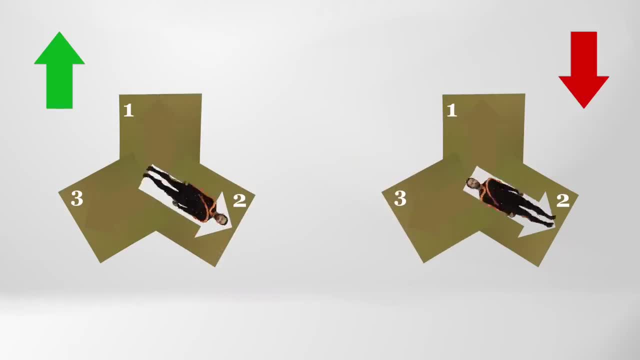 and the only criterion that plan must satisfy is that if the particles are ever measured in the same direction, they must give opposite spins. So, for example, one plan could be that one particle will give spin up for every measurement direction and its pair would give spin down. for every measurement direction Or another plan. plan two could be that one particle could give spin up for the first direction, spin down for the second direction and spin up for the third direction, Whereas its partner would give spin down for the first direction. 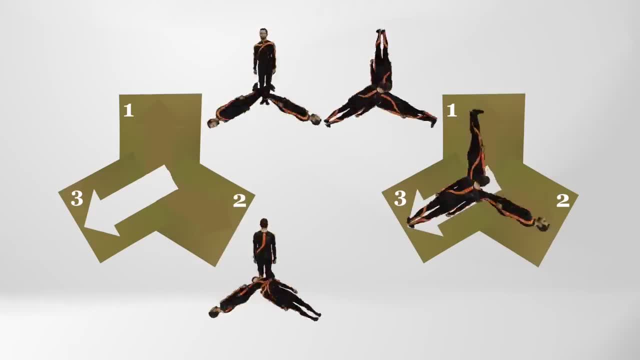 spin up for the second direction and spin down for the third direction. All other plans are mathematically equivalent, so we can work out the expected frequency of different results using these two plans. Here I'm visually representing the particles by their plans. 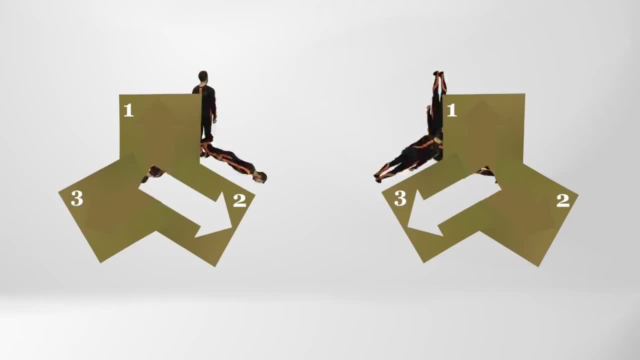 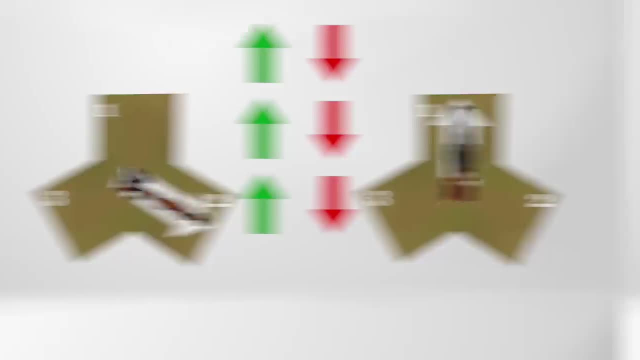 their hidden information. With plan one, the results will obviously be different. 100% of the time. It doesn't matter which measurement directions are selected, But it does for particles using the second plan, For example, if both detectors measure in the first direction. 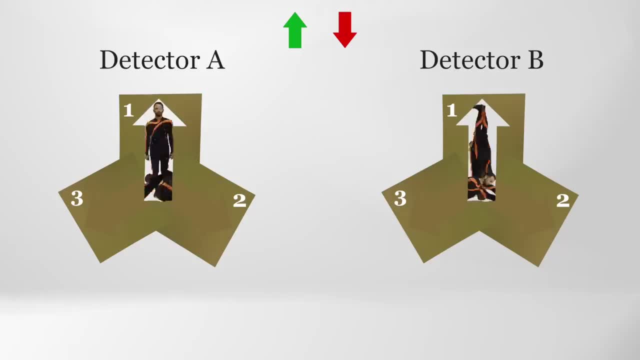 particle A gives spin up while particle B gives spin down, The results are different. But if instead, detector B measured in the second direction, the result would be spin up. so the spins are the same. We can continue doing this for all the possible measurement combinations. 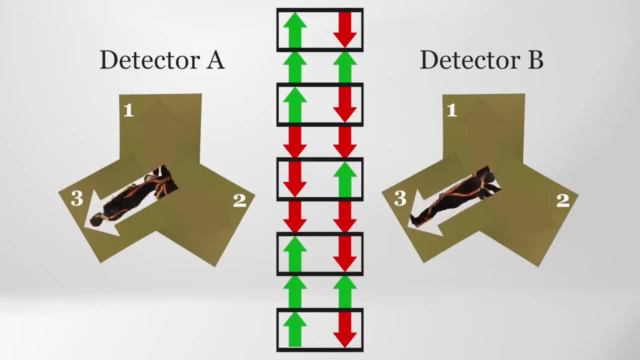 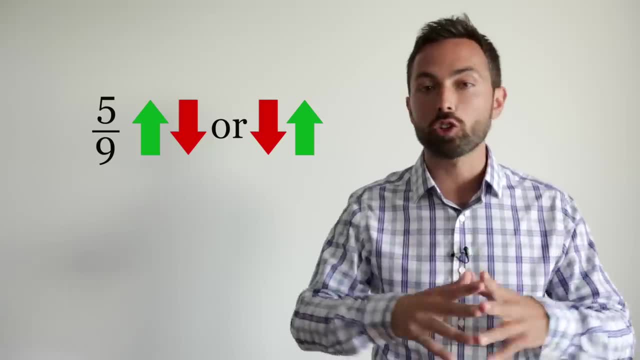 and what we find is the results are different five out of nine times. So, using the second plan, the results should be different five-ninths of the time, And using the first plan, the results should be different 100% of the time. 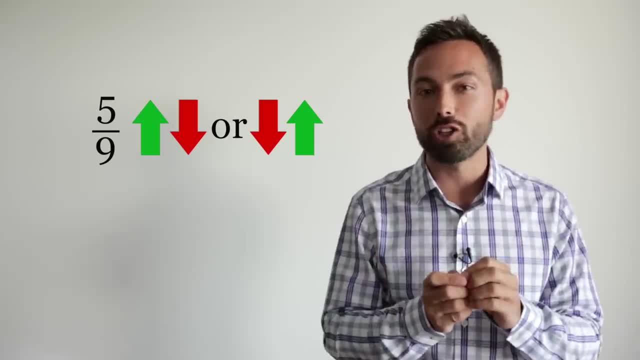 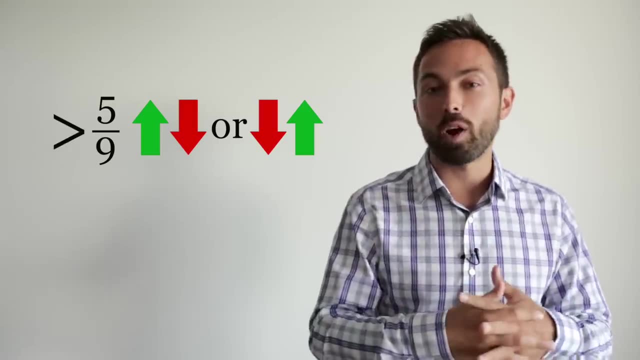 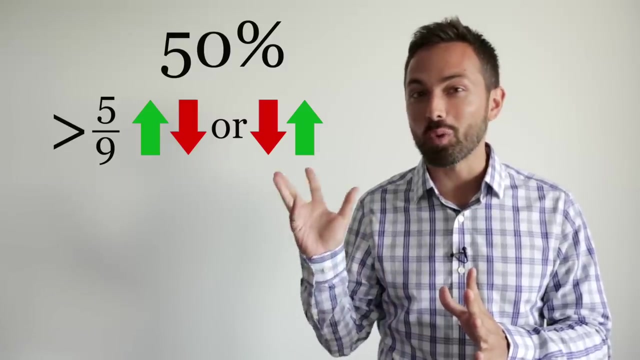 So, overall, if the particles contain hidden information, you should see different results more than five-ninths of the time. So what do we actually see in experiment? Well, the results are different only 50% of the time. It doesn't work. 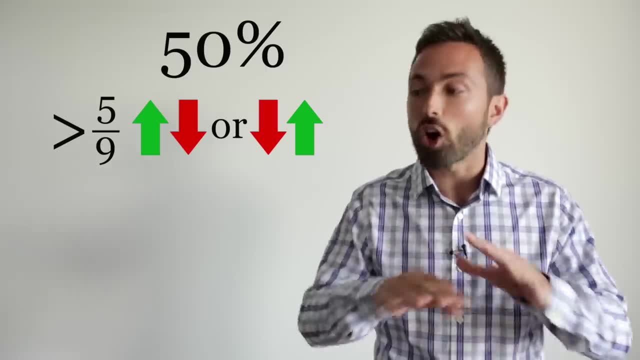 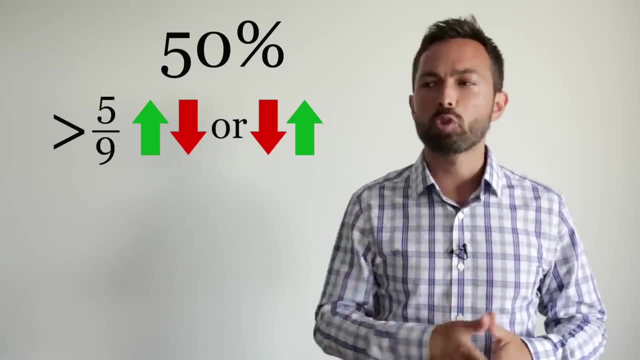 So the experiment rules out the idea that all along these particles contain hidden information about which spin they will give in the different directions. So how does quantum mechanics account for this result? Well, let's imagine detector A measures spin in the first direction. 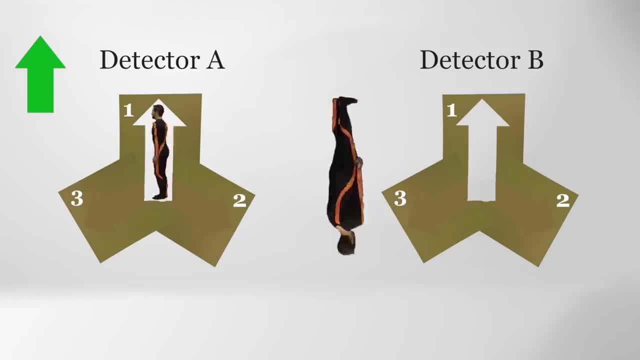 and the result is spin up. Now, immediately, you know that the other particle is spin down if measured in the first direction, which should happen randomly one-third of the time. However, if particle B is measured in one of the other two directions, 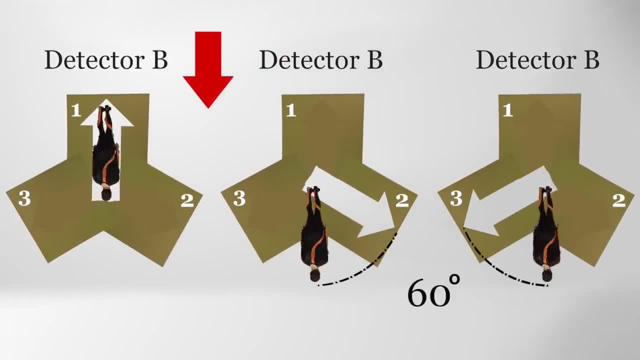 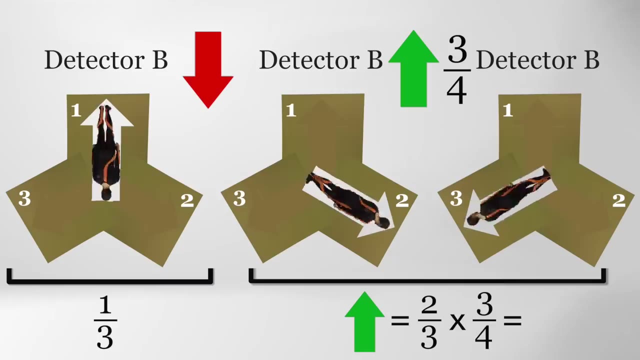 it makes an angle of 60 degrees with these measurement directions And recall from the beginning of this video- the resulting measurement should be spin up three-quarters of the time. Since these measurement directions will be randomly selected two-thirds of the time particle B will give: spin up two-thirds times three-quarters equals half of the time.